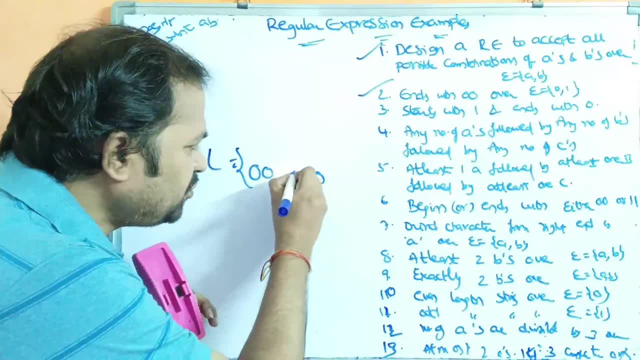 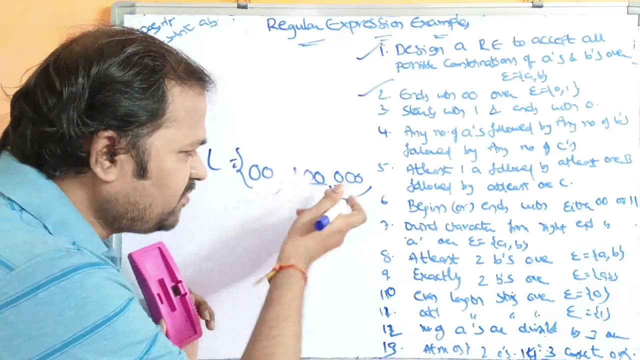 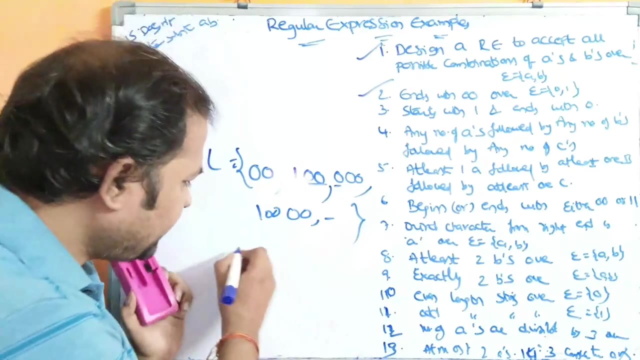 It ends with zero zero, So before zero zero, we can have any number of zeros and ones. It ends with zero zero, So before this we can have one. Before this, we can have one. Before this, we can have any number of zeros and ones. There is no constraint on that. So the regular expression for this is: 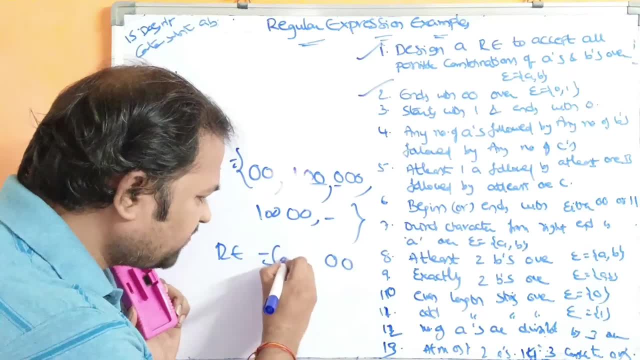 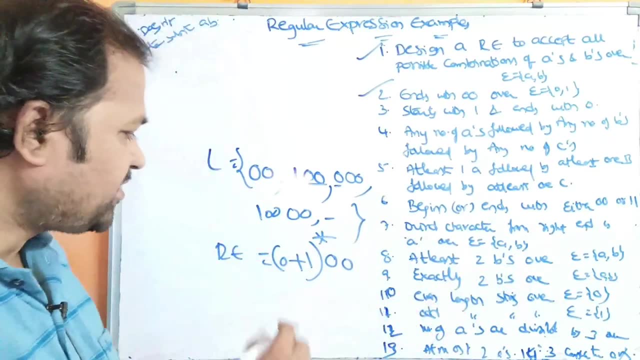 ends with zero zero. So before zero zero, we can have any number of zeros and ones. So before zero zero, we can have any number of zeros and ones. So this can be written as zero plus one whole star, zero, zero, Okay, Any combinations of zeros and ones. Next one starts with one and ends. 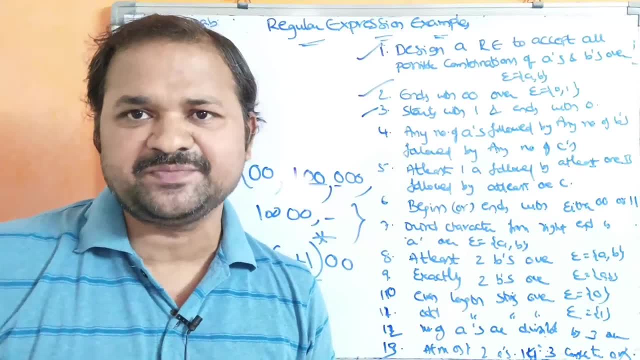 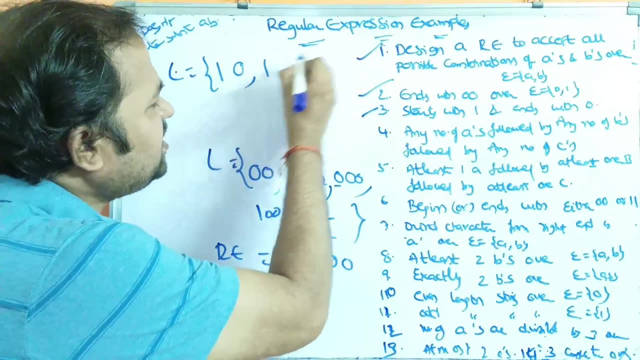 with zero. So here also, the input alphabet contains two symbols: Zero and one. Here what is the language? The language starts with one and ends with zero. So in between one and zero we can have any number of zeros and ones. So there is no constraint on that. So let 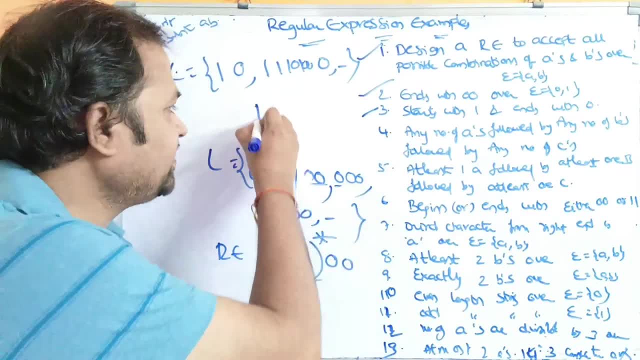 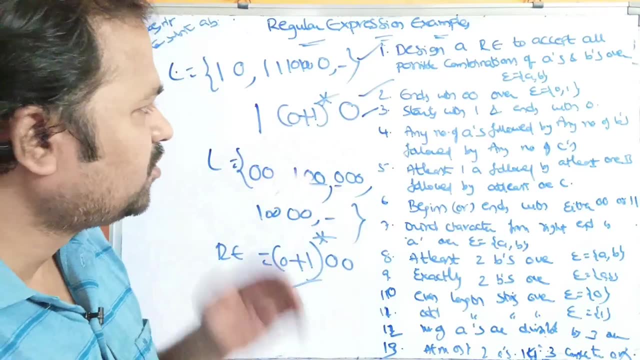 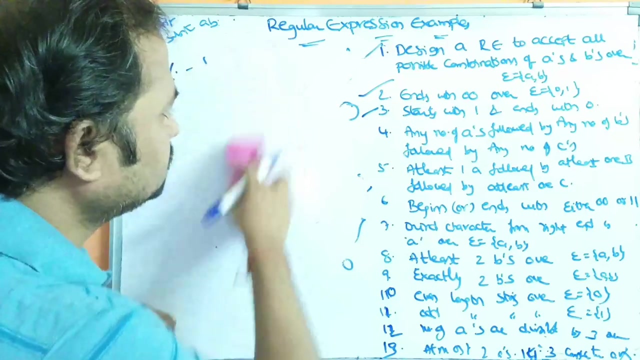 us design the regular expression So it starts with one Okay And ends with zero. So in between we can have any number of zeros and ones. So zero plus one whole star. Now let us see the next example. Let us see the next example. Fourth one: Any number of a's followed by any number of b's. 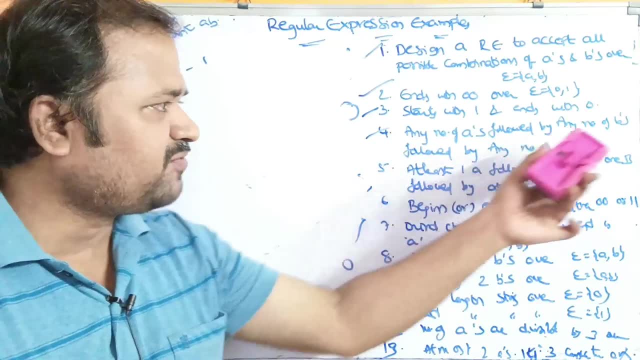 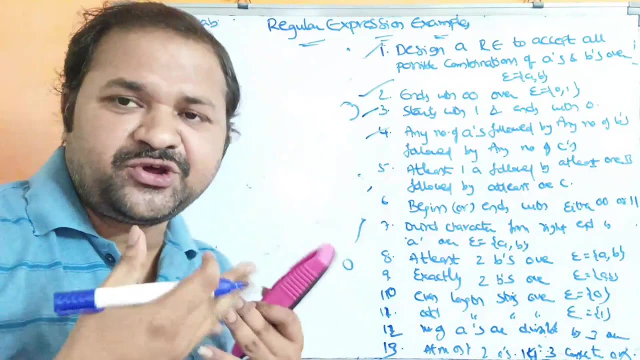 followed by any number of c's. So here the input alphabet majorly contains three symbols: a, b, c. So what is the language here? L is equal to. You may have zero number of a's, zero number of b's, zero number of c's. 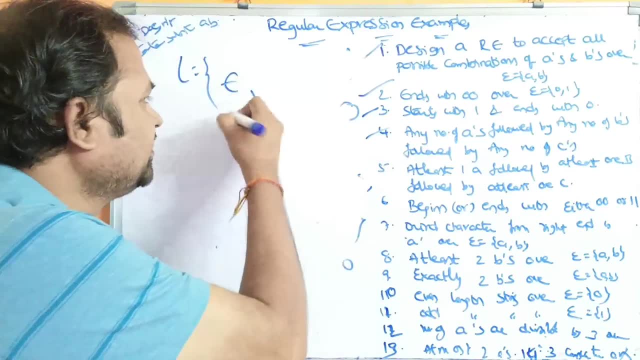 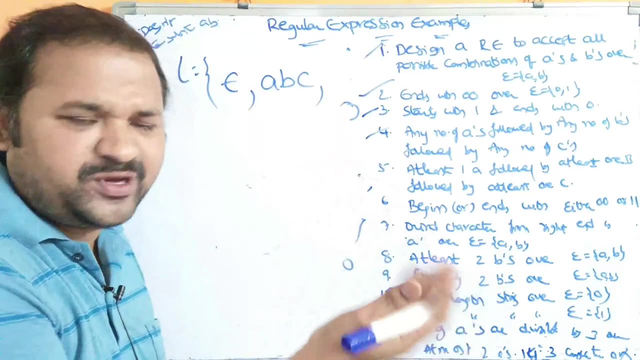 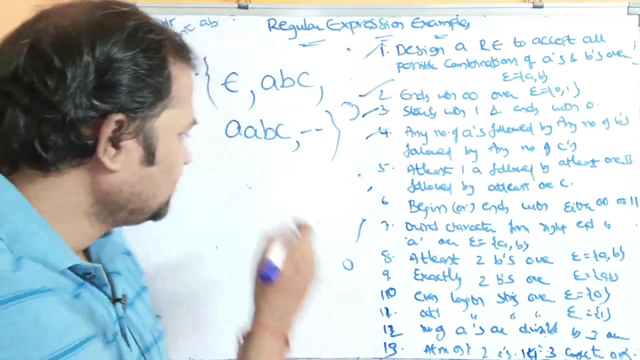 also So that can be represented by epsilon. Next, let us assume that one a is followed by one b is followed by one c, So a, b, c, We can have two a's. So two a's are followed by single b, single c. Likewise we can write n number of strings. So the regular expression. 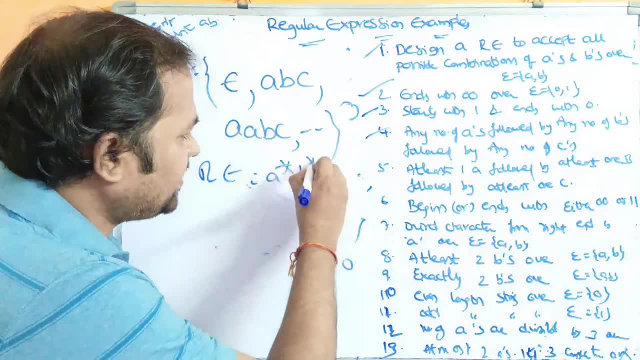 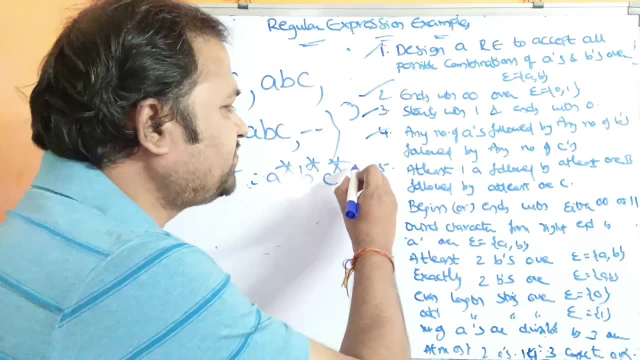 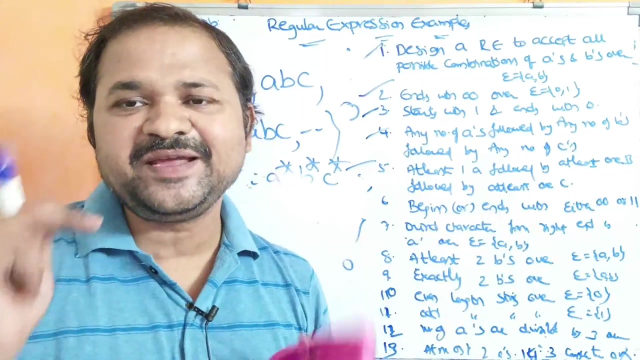 for this is a star, b star, c star, Any number of a's followed by any number of b's, followed by any number of c's. Now let us see the next one: At least one a, followed by at least one b, followed by at least one c. So that means: 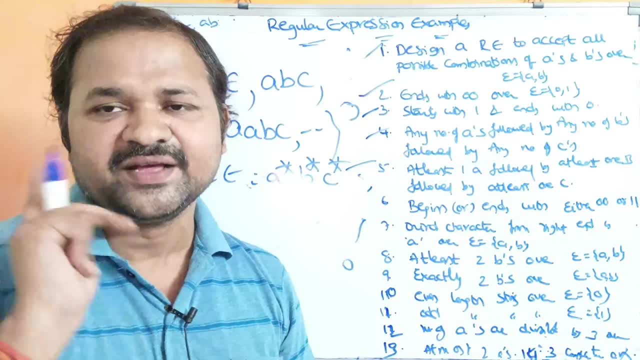 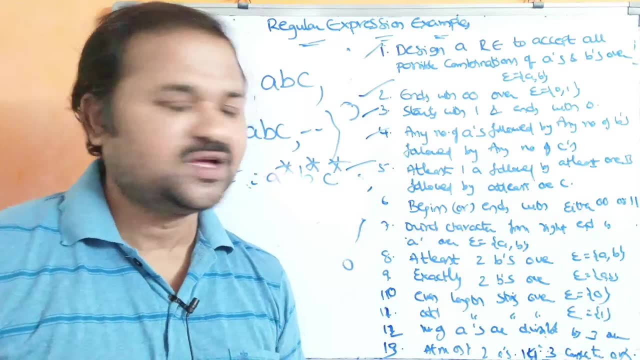 zero occurrence is not possible. We should have minimum one a, minimum one b, minimum one c. So that means epsilon is not there, So that the remaining strings are as it is Okay. Now in place of the star we can write plus. So plus means positive closure, So positive closure. 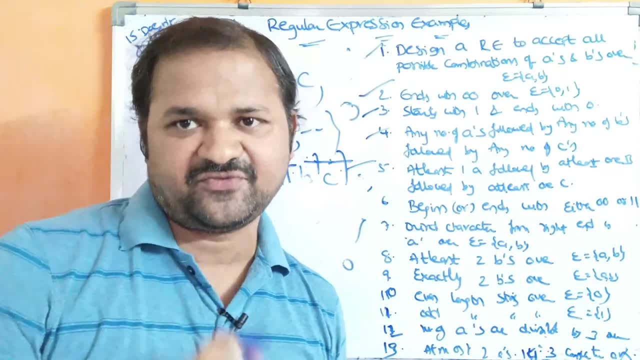 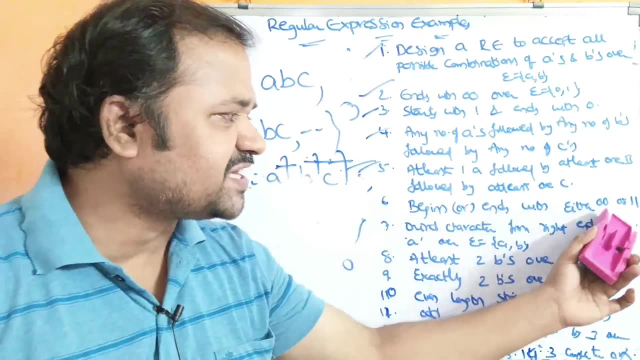 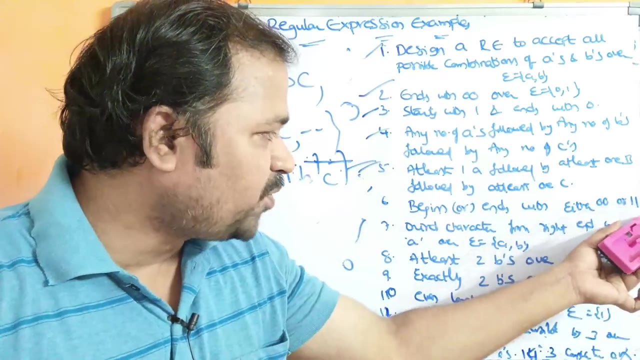 means zero occurrence is not possible, So we should have minimum one occurrence: A plus b plus c plus. Now let us see the next. one Begins or ends with 0, 0 or 1, 1.. So here the corresponding string may begins with 0, 0 or the corresponding string may begins with 1. 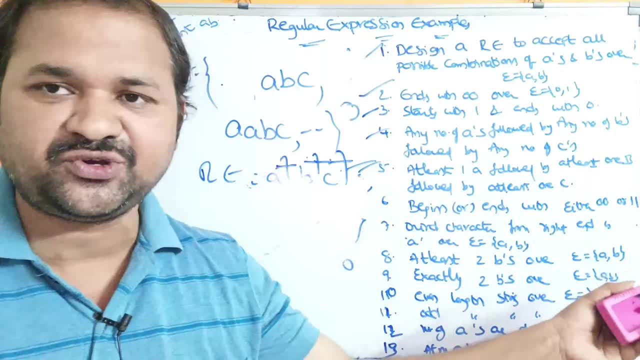 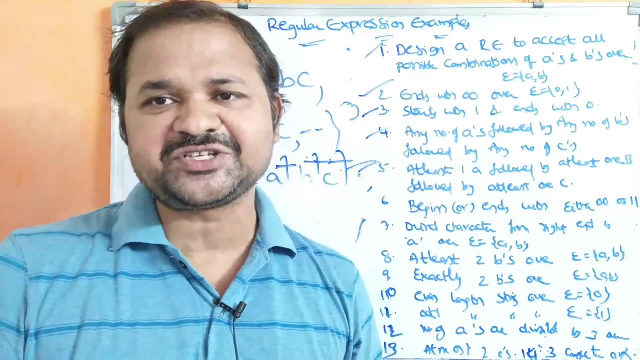 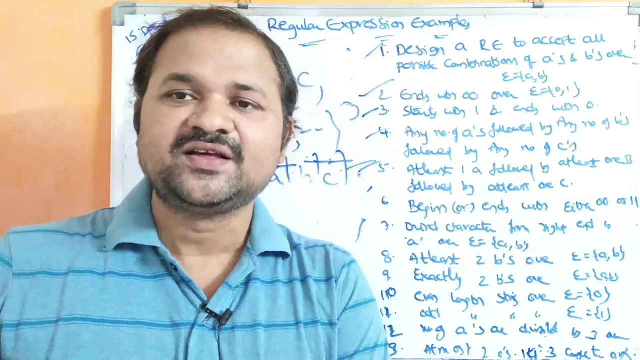 1, or the corresponding string may ends with 0: 0, or the corresponding string may ends with 1: 1.. So, totally, here we have four combinations, are there? What is the first combination? The strings starts with 0: 0.. Second combination: the strings starts with 1: 1.. Third combination: 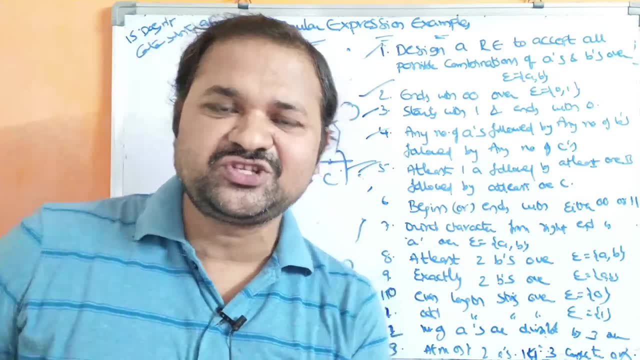 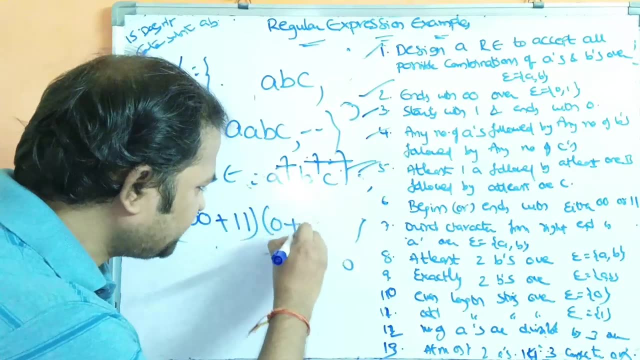 strings ends with 1: 1.. Next strings ends with 0: 0. So this can be written as so: 0, 0 plus 1: 1 into 0 plus 1 whole star. So this combination means the corresponding string may. starts with: 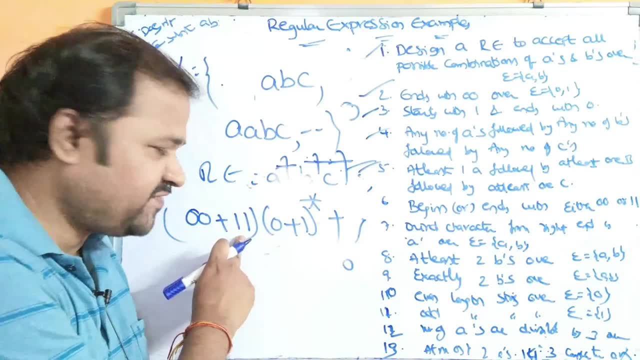 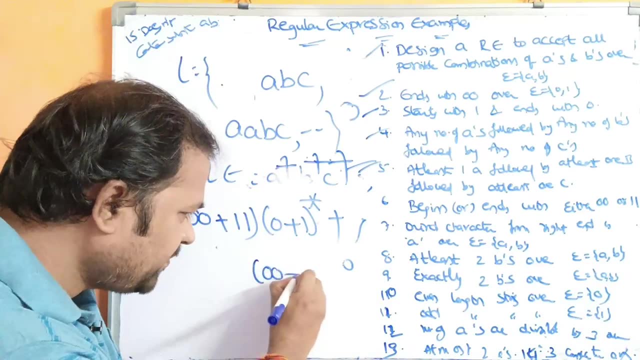 0, 0 or the corresponding string may starts with 1, 1.. After that, we can have any number of 0's and 1's. And what is the second combination? The corresponding string may ends with 0, 0 or the corresponding. 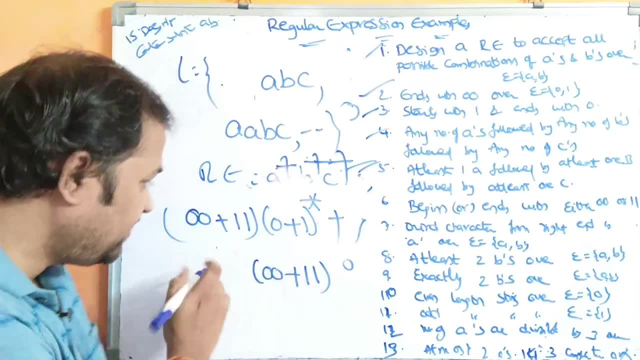 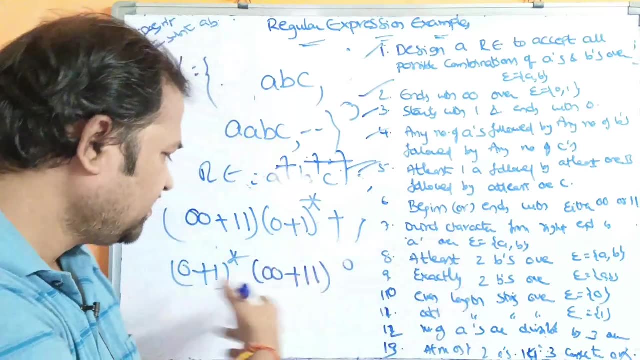 string may ends with 1- 1.. So before this, 0, 0 and 1- 1, we can have any number of 0's and 1's. So this is the language, This is the regular expression. So for this one According: 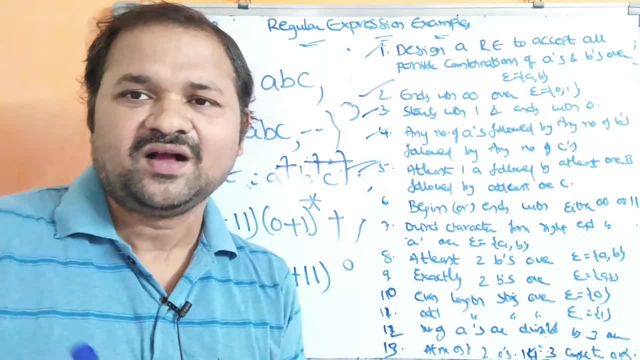 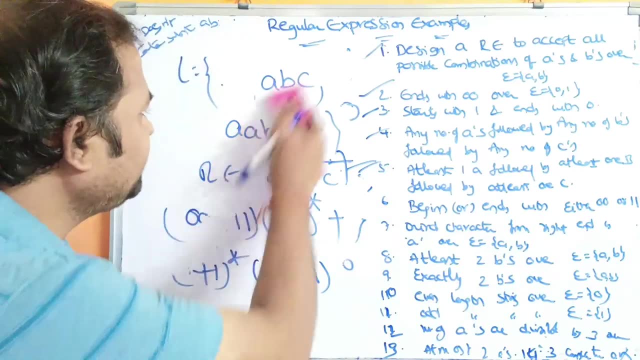 to that. we can write the language: 0: 0 comma. 1, 1 comma. Before 0: 0, we can have any number of 0's and 1's. After 0: 0, we can have any number of 0's and 1's According to that you. 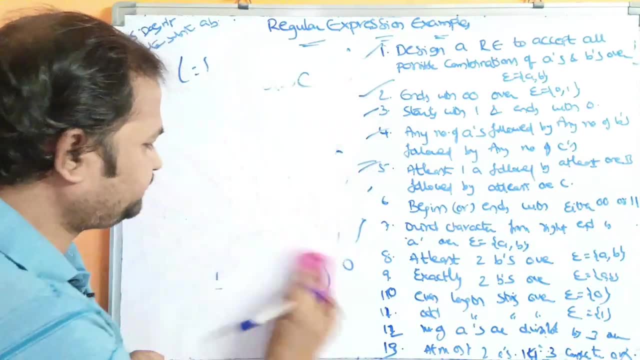 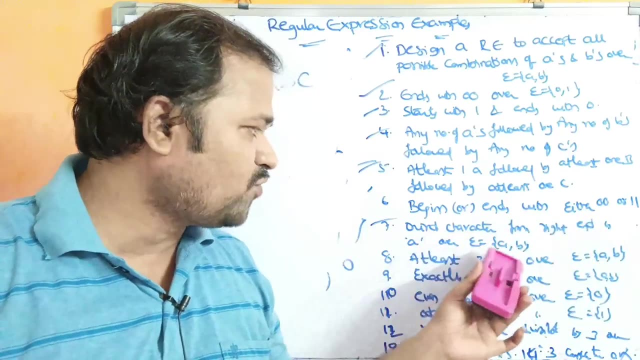 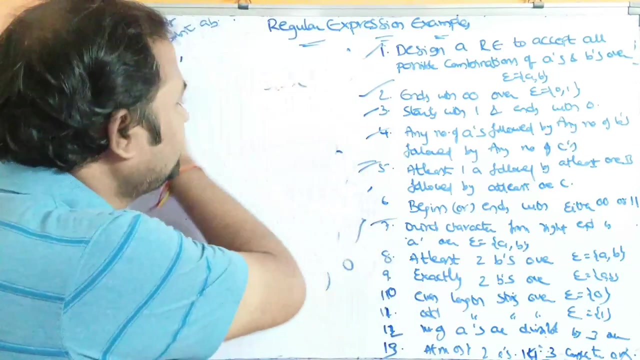 can write the language. Now let us see the next example. What is the next example? Seventh example: Third character from the right end is a. over sigma is equal to a, comma, b. So third character from the right end is a. So this is the first character from the right end, So this character may. 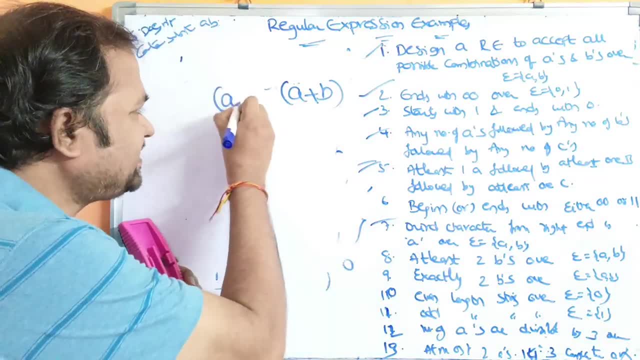 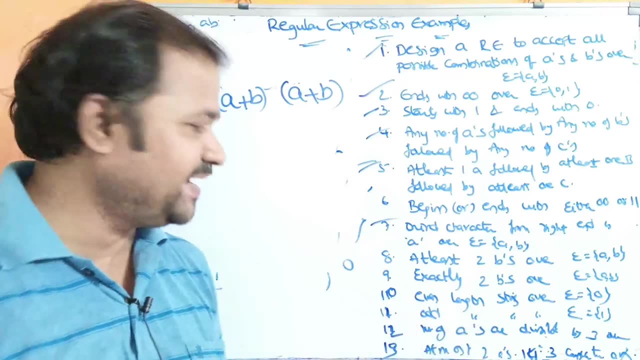 be either a or b, And this is the second character from the right end. This character may be either a or b, Why? Because here the input alphabet contains two symbols. They are the first letter, a and b, Whereas the third character from the right end is a. So this is the third. 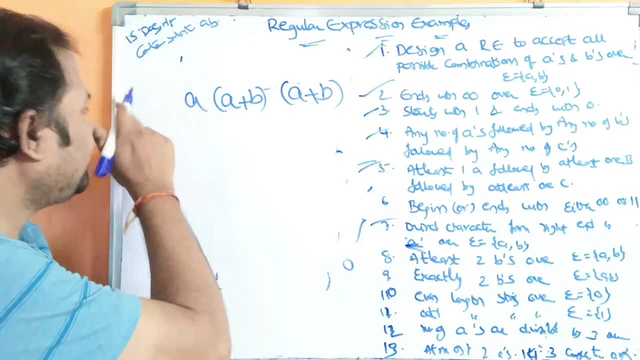 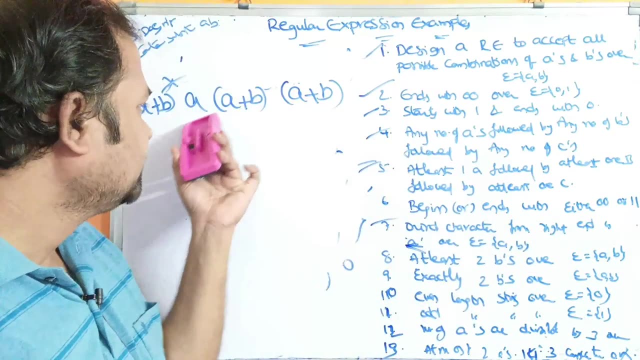 character from the right end. It should be a only, So after this we can have any number of a's and b's. So there is no constraint on that. Third character from the right end is a. So this is the first character. It may be either a or b. It is the second character. 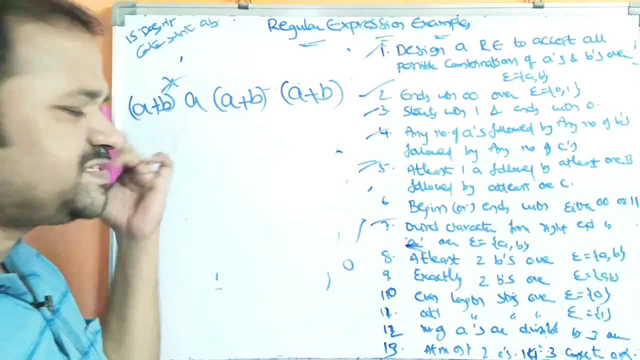 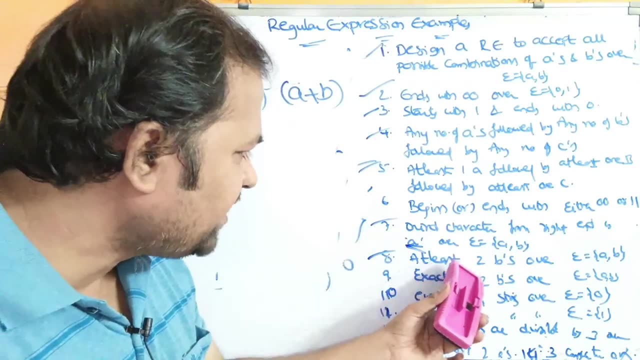 It may be either a or b. Third character is a, And before this we can have any number of a's and b's. Let us see the next example: Design. a regular expression for at least 2 b's over sigma is equal to a comma b. here the regular expression should: 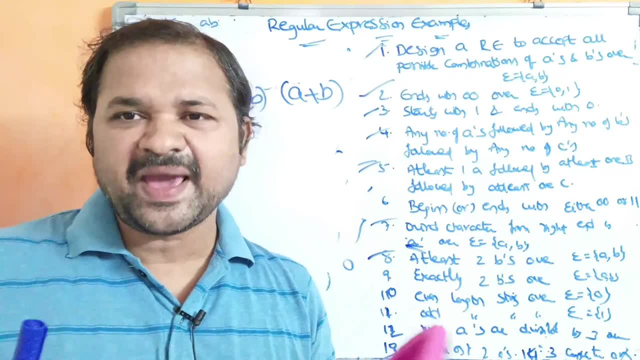 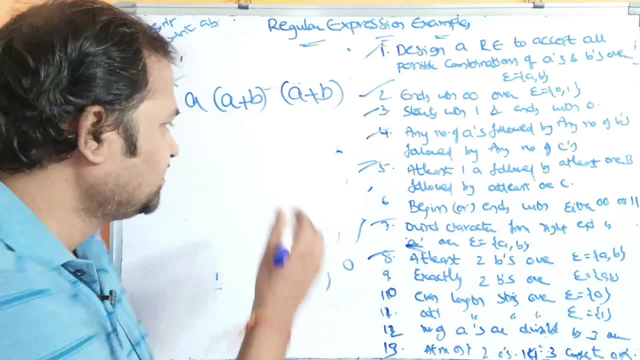 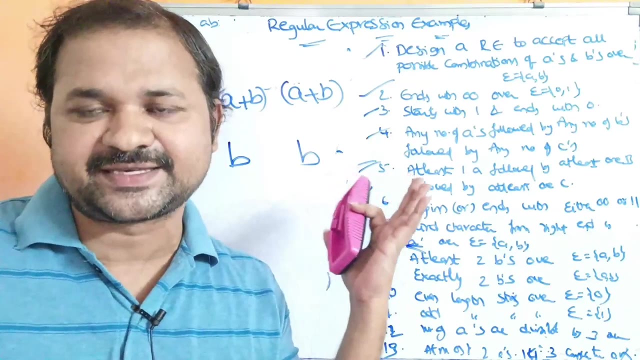 contain minimum 2 b's. what about maximum? maximum may be any number, there is no constraint on that, but the corresponding regular expression should accept minimum 2 b's. so minimum 2 b's, minimum 2 b's, and we can have any number of a's and b's. there is no constraint on that, so we can write. 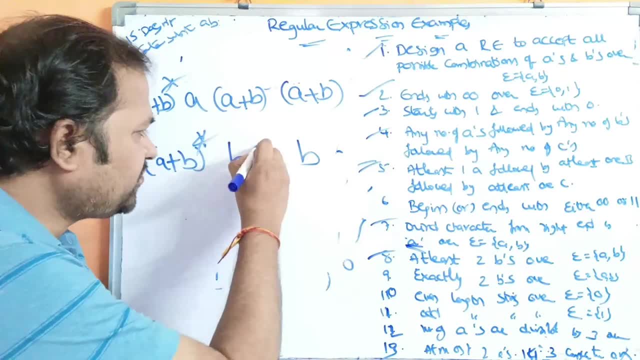 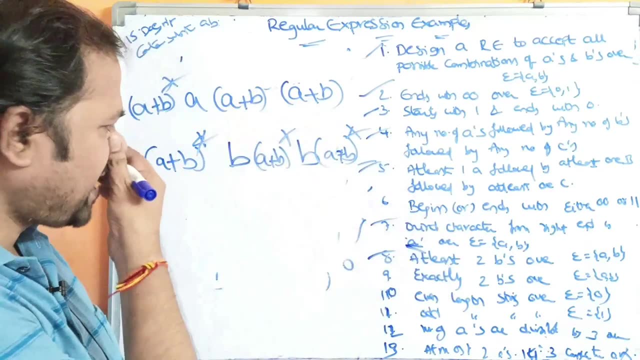 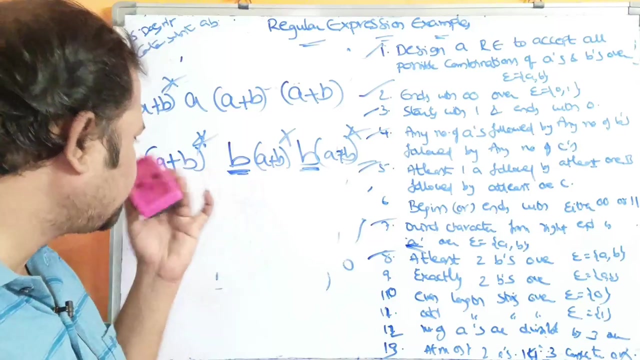 as a plus b whole star. here also a plus b whole star, a plus b whole star. so the corresponding language accept strings which contains minimum 2 b's maximum. there is no constraint on that. so before this b, any number of a's and b's. after this b, any number of a's and b's after this b: any. 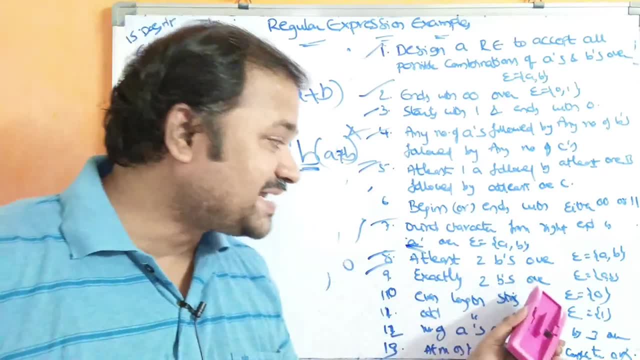 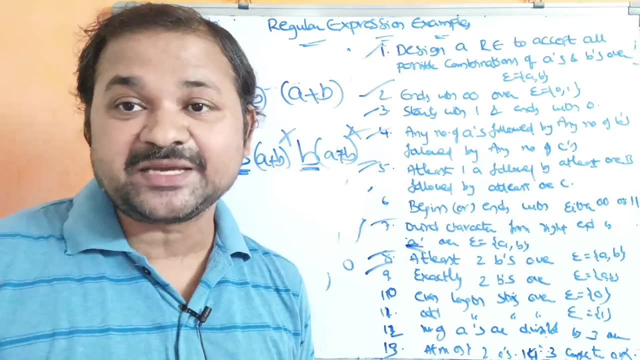 number of a's and b's. let us see the next example. exactly 2 b's over sigma is equal to a comma b. the corresponding language, the corresponding regular expression should accept only 2 b's, so only 2 b's. so before this we can. 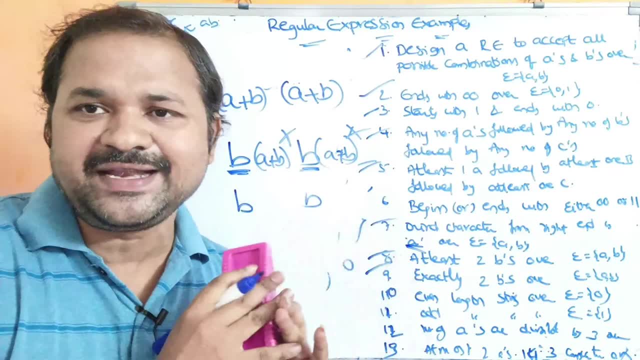 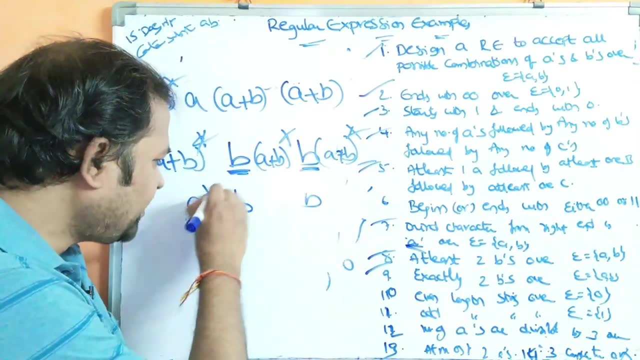 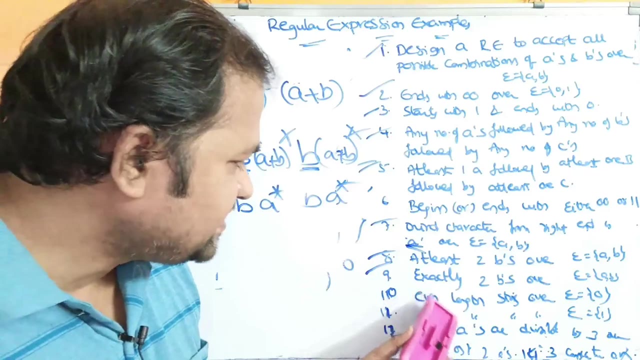 have any number of a's, but it should not contain b's. why? because it should. it should accept only 2 b's only, so there is no constraint on number of a's. there is no constraint on number of a's, but we should not have any b's here. okay, let us see the next one. even length. string over sigma. 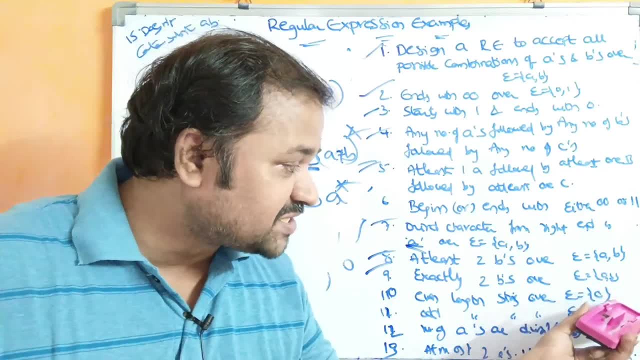 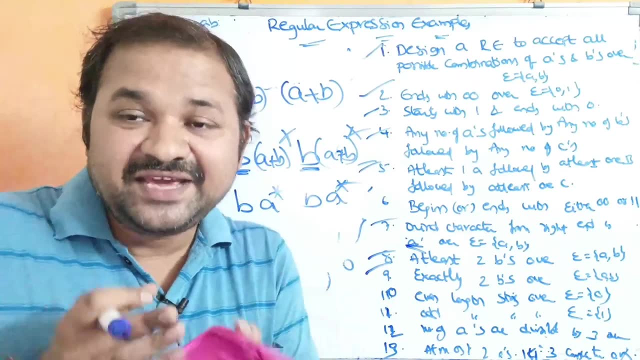 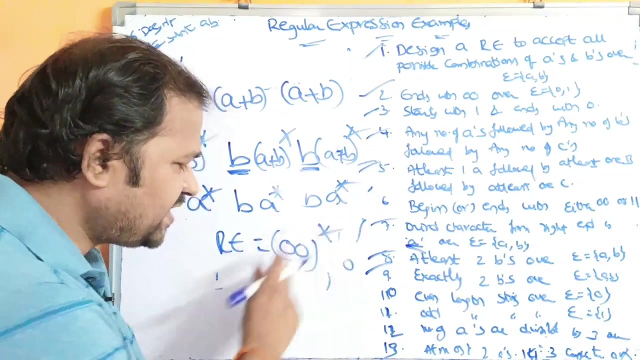 is equal to zero. here the input alphabet contains zero, so here even length means it may be zero also. okay, so epsilon comma, zero, zero, comma even length means two, four, six, eight, like that. okay, so we can write regular expression as zero, zero, whole star. so one occurrence means epsilon, zero occurrence means 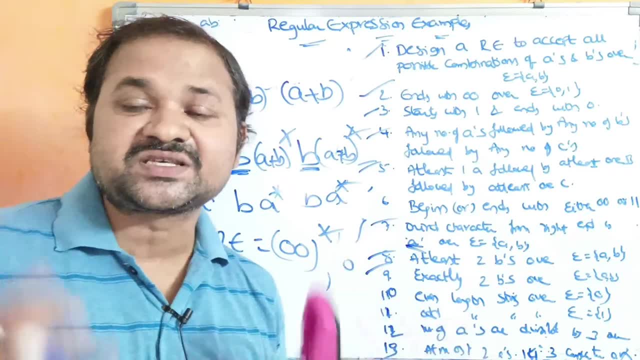 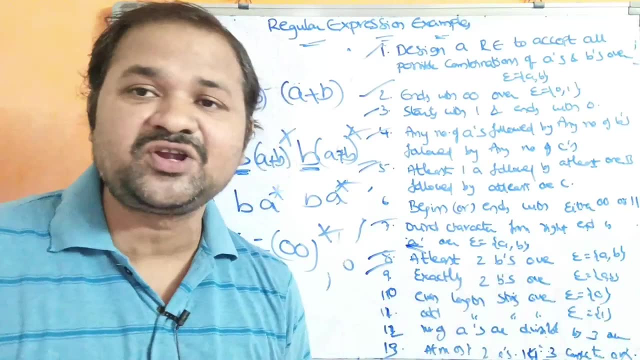 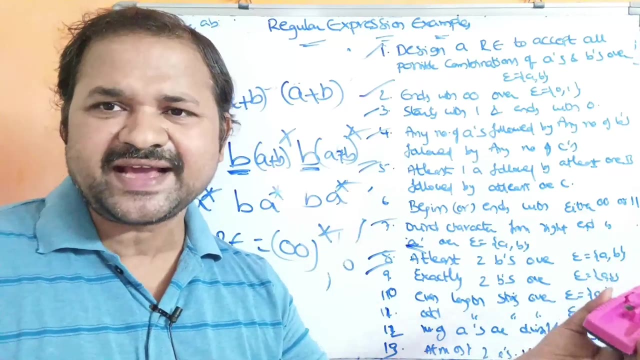 epsilon: one occurrence means zero zero. two occurrence means four zeros. three occurrence means six zeros. likewise. next, one odd length strings over sigma is equal to one. so what is odd length string? one comma three bull. one comma five ones comma. it should not accept epsilon. so one comma three, three. one comma, five ones comma. why? because odd length string over. 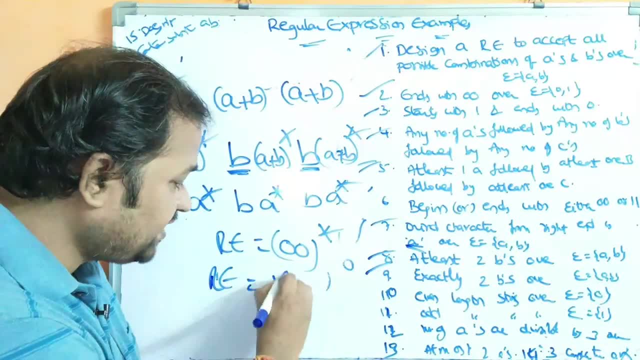 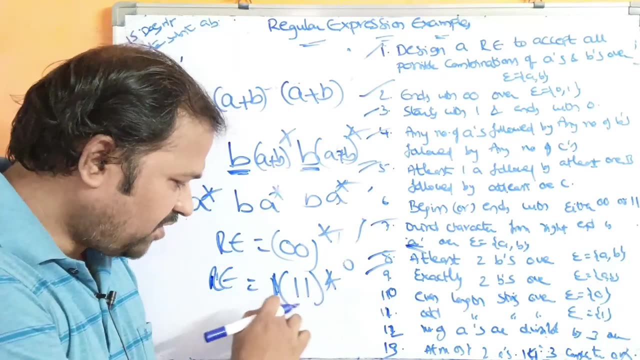 sigma is equal to one, so we can write this as one into one, one whole star. so if we have one zero occurrence of this combination, one one, then what will happen? one into epsilon means one. if we have one occurrence of one one, then triple one. if we have two occurrence, 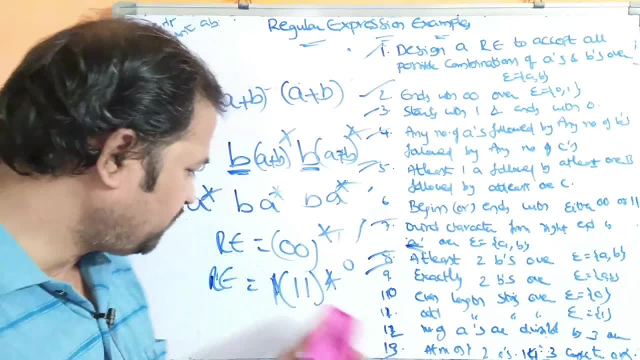 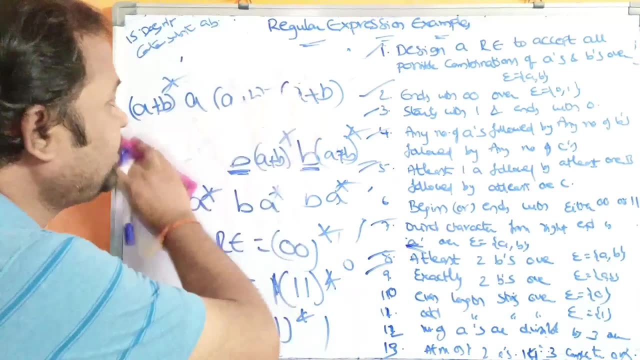 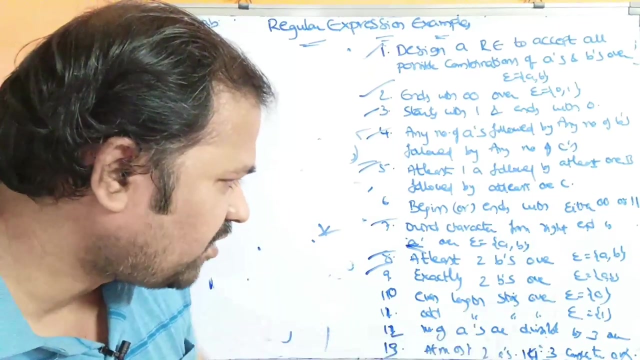 two, two, one. two occurrence means what? four, one. so four one into one means five, one. or we can write this as like this: also: one, one, whole star, one. after this also we can write: now let us see the remaining examples. so what is the next one? number of a's are divisible by three, so number of a's are: 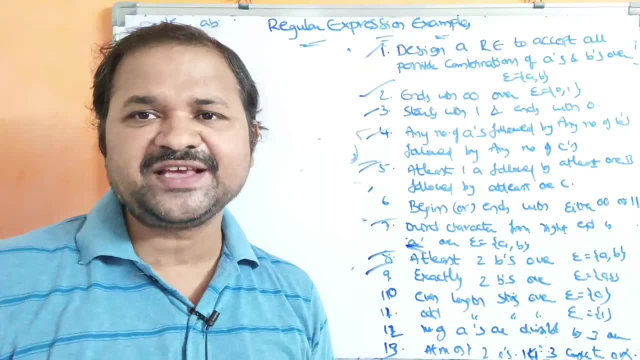 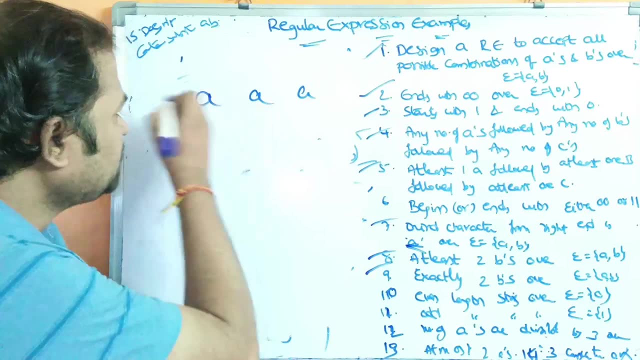 divisible by three. so a's may be either zero number of a's or three a's, or six a's, or nine a's or twelve a's, like that. so number of a's are divisible by three. so number of a's are divisible by three. so before this we can have any number of b's, so there is no constraint on that. so we can. 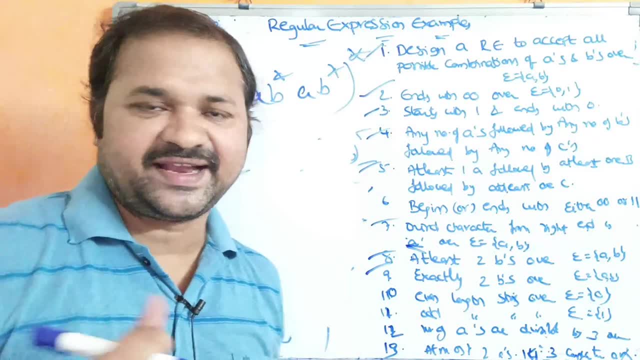 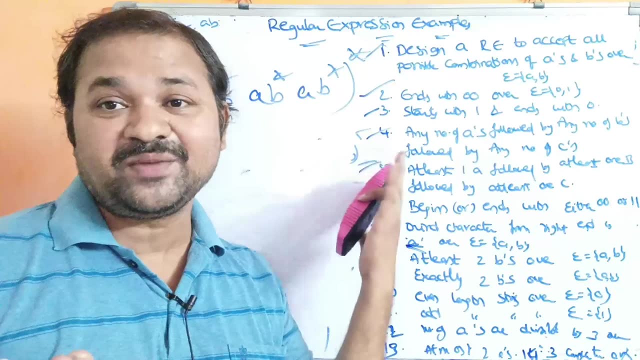 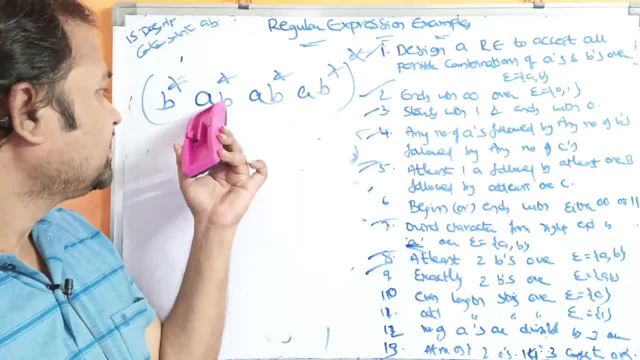 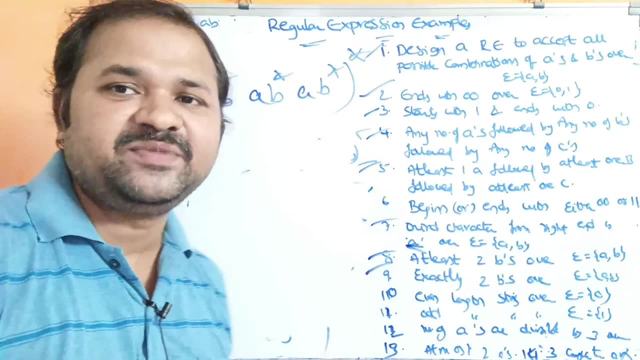 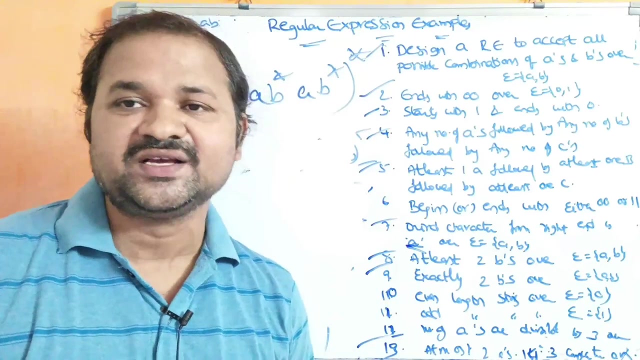 a's. if you take two occurrence, then we will get a. a is written two times, so two a two a two a means six a's. so if you write three, three a three a three a means nine a, so likewise we will get- let us see the next example- at most two a's, at most two a's, so here we can have maximum two a's. 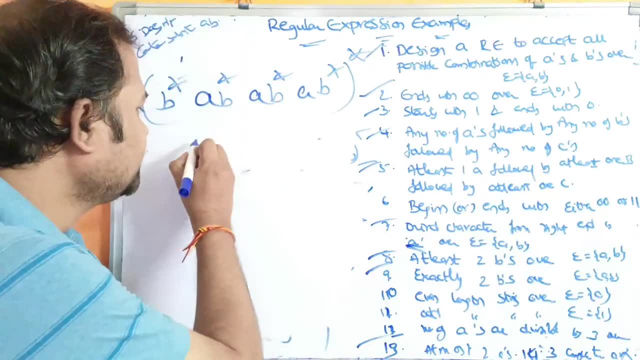 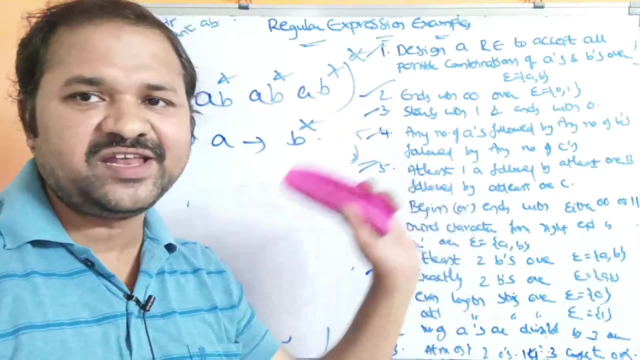 so that means zero a or one a or two a. so zero a means we can write as b star, because it doesn't accept any a's. we can have any number of b's. one a means we can write as one a, so before this we can have any number of b's. 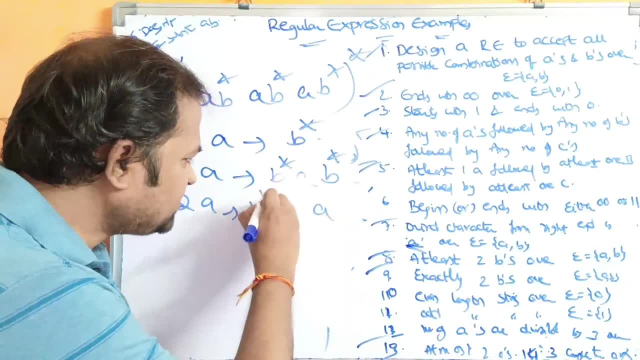 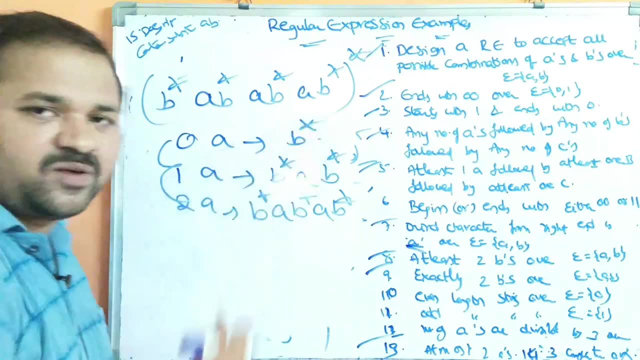 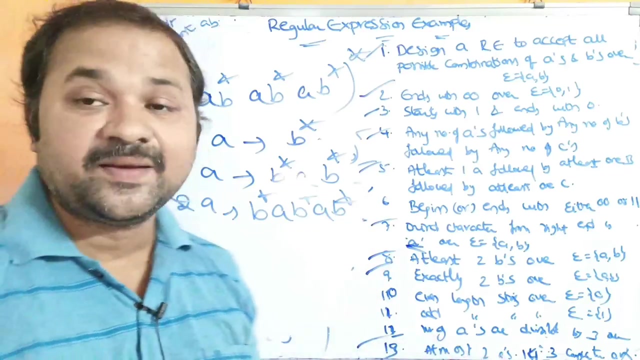 if we write two a, then two a, so before this we can have any number of b's. okay. next, at most at most two a's means we have to add all these terms, so b star plus b star, a b star plus b star, a b star, a b star at most means what? maximum two a's so we may have zero a. zero a means this will: 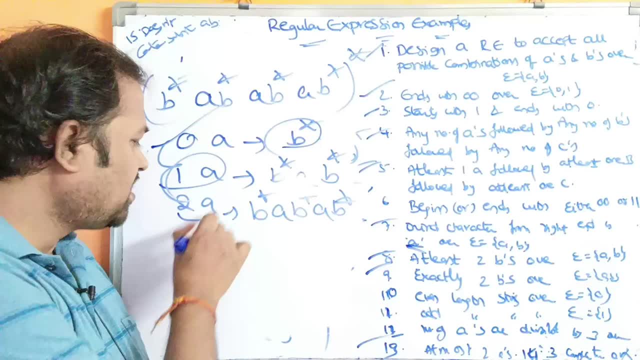 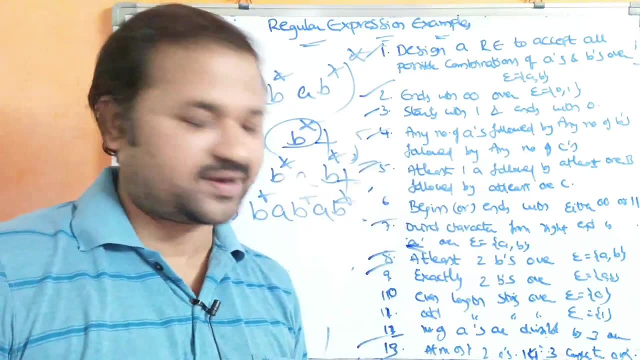 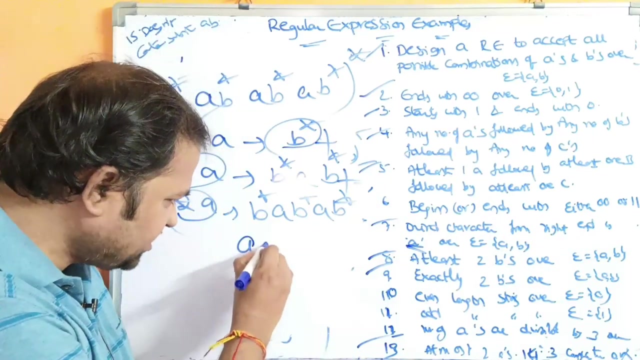 be accepted. or one a, it will be accepted, or two a means this will be accepted. we have to use r. r or this plus symbol is nothing but r. and the next one is three consecutive a's. three consecutive a's, so here we have three consecutive a's. so before this, these a's, we can have any number of a's, and 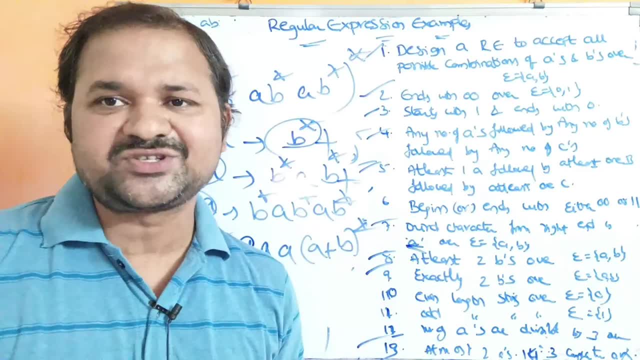 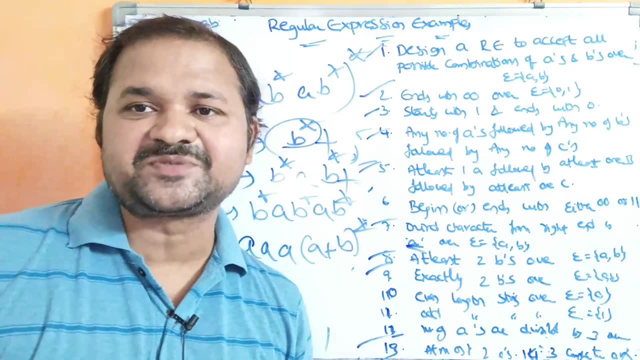 b's. after this, we can have any number of a's and b's. there is no constraint on that. let us see: the last example doesn't contains the substring a- b. it doesn't contains the substring a- b. for this the answer is regular expression: is b star a's? 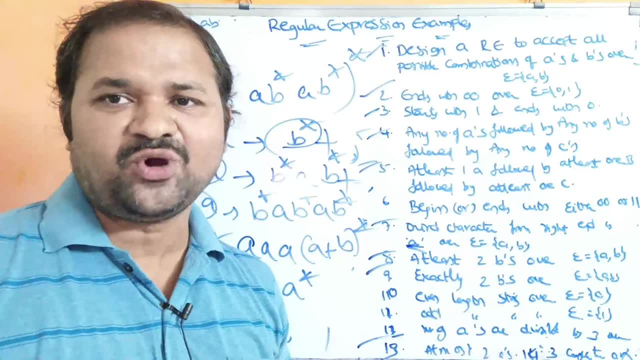 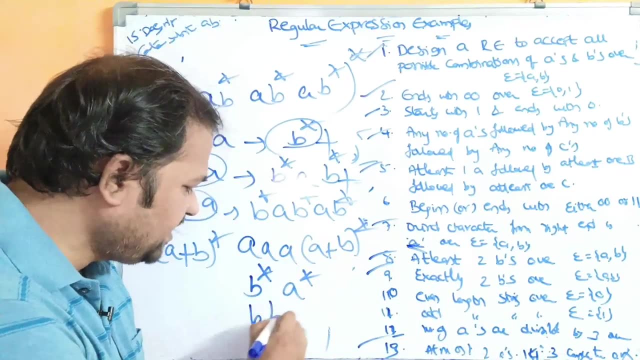 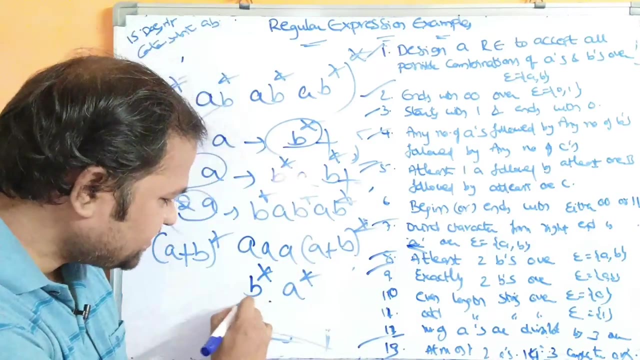 b star. a star doesn't contains a- b. if you take zero occurrence, then we will get b- a, so it doesn't contains a- b. if you take two occurrences, then we will get b, b, a, a. so here this one doesn't contains the substring a- b if you take three occurrence. if you take two occurrences of b. 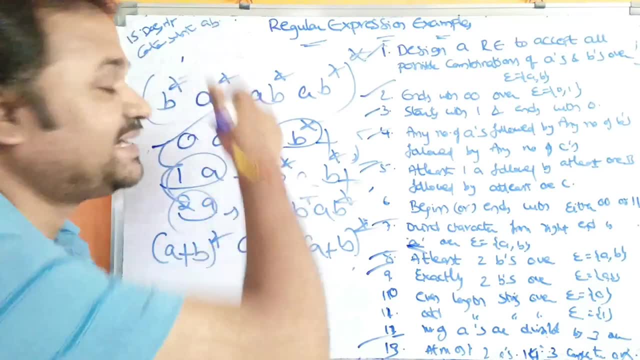 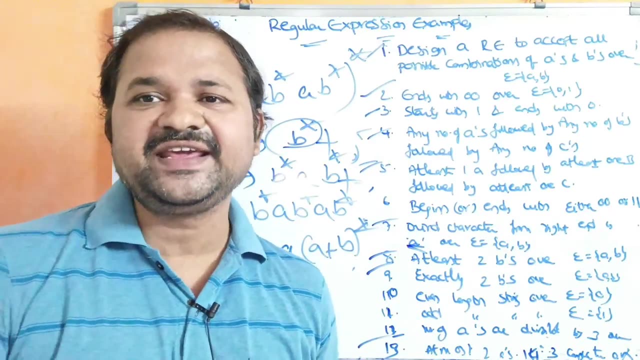 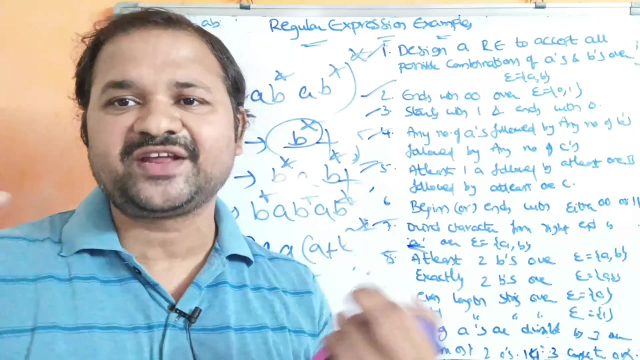 and one occurrence of a, so b, b, a. it doesn't contains a, b, so in this way we can solve any problem regarding the regular expression very, very easily. so this is about regular expression examples: designing a regular expression for a given problem.